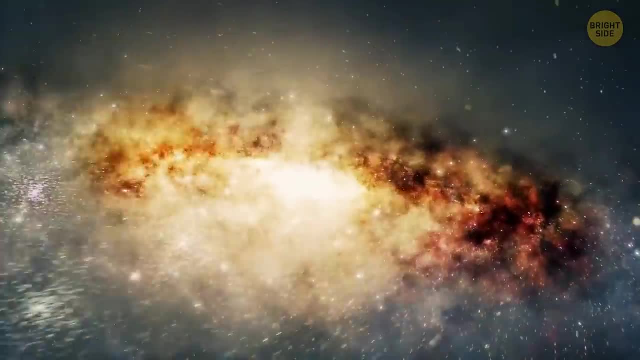 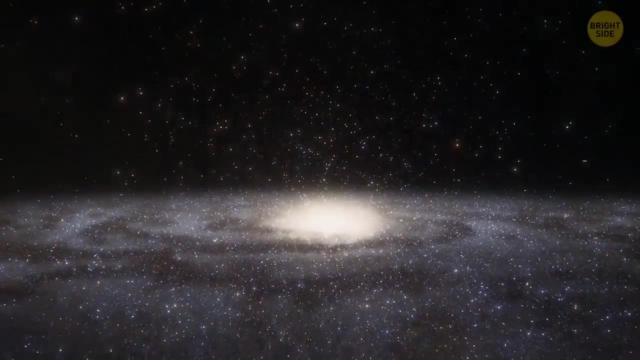 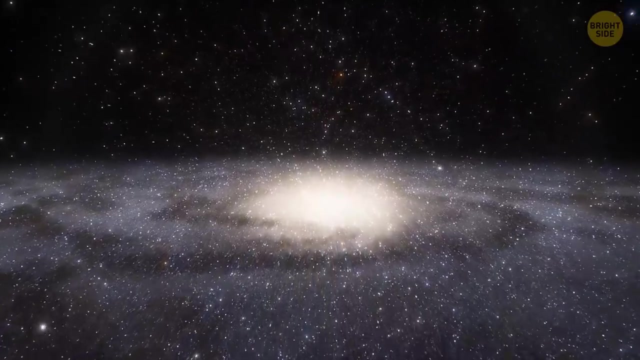 How was our universe born? And if this seems hard to answer, then how about this? What was before our universe? While scientists are looking for the answer to the most difficult question in history, let's find out what they've come up with so far. 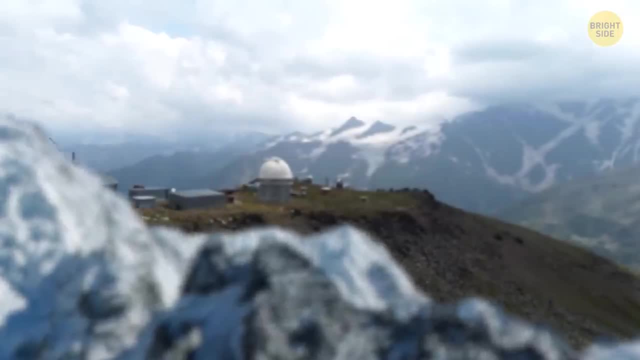 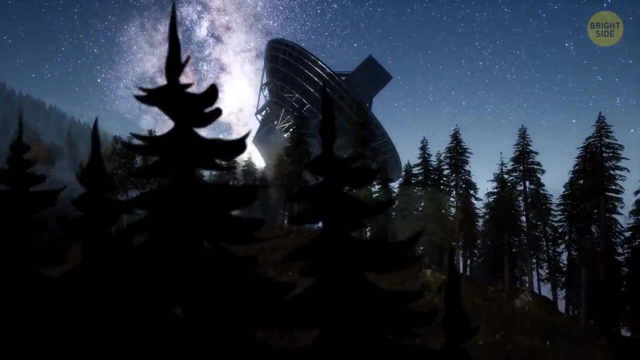 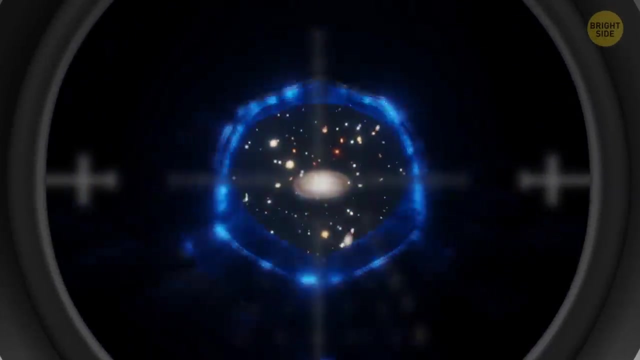 In the 20th century. we've shed the light on this mystery, all thanks to this man, Edwin Hubble. One day on Mount Wilson in Southern California, he aimed his telescope at the sky and found out that these random clouds of gas flying everywhere are actually other galaxies- and there are a lot. 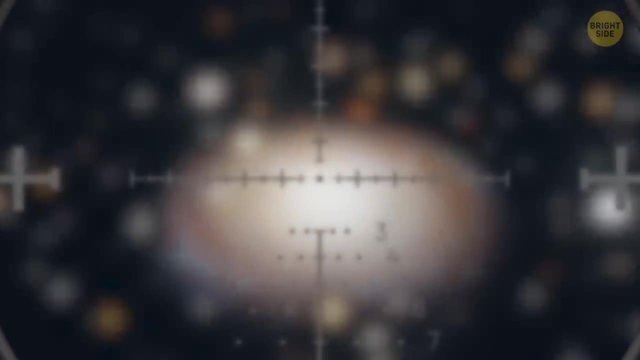 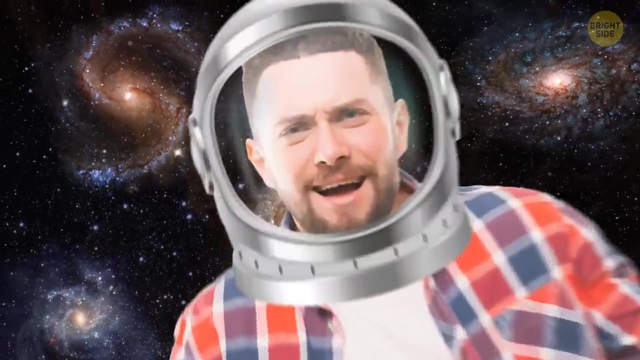 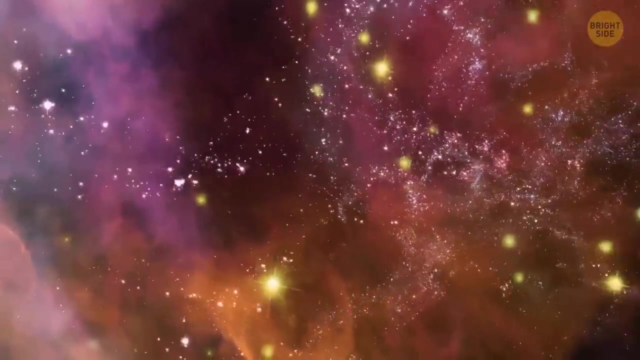 of them. And also he learned something else, something that changed the world forever. They're moving. So what you may ask? Well, it meant one very important thing: The universe is expanding, and if it's expanding, then it probably had a beginning somewhere. right Now, all we have to do is run time backwards. 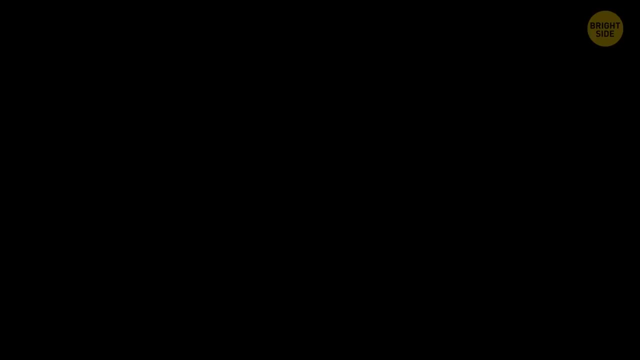 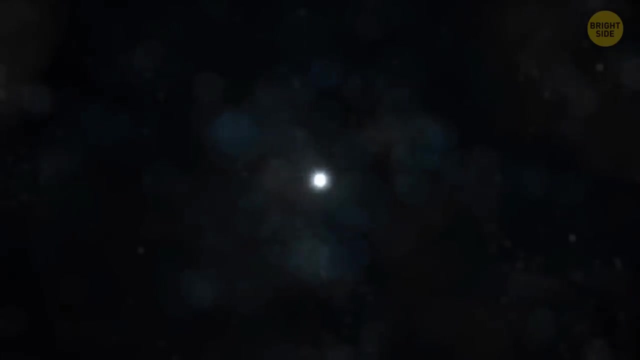 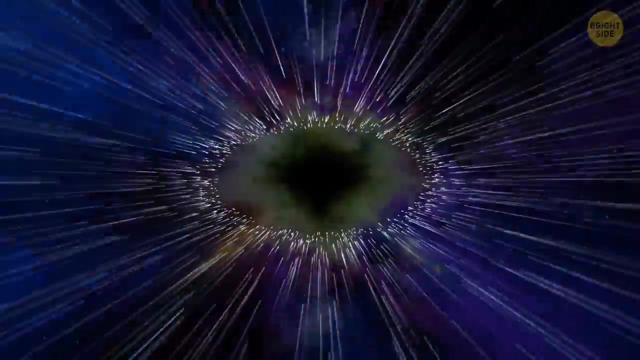 and see where the beginning was. It took the scientists many more years to come up with a full-fledged theory, the Big Bang Theory. And here it is. Nothing has ever been anywhere because neither when nor where existed. Do you get it? But actually no, There was one thing. 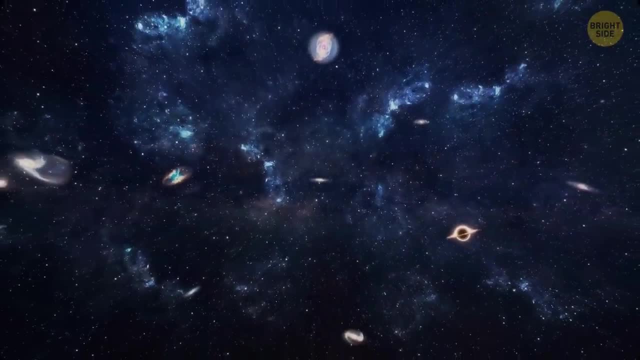 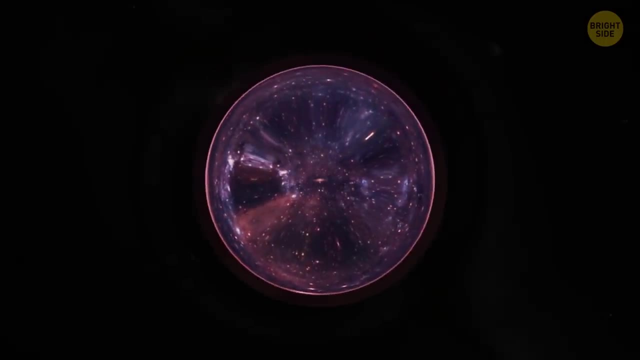 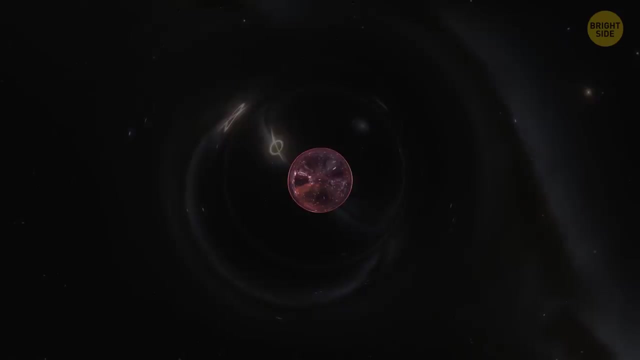 It was the so-called cosmopolitan. It was the so-called cosmopolitan, the cosmic singularity, A state of our universe in which it was incredibly small, dense and very hot. Imagine if our universe was compressed into a small ball. The pressure and temperature inside would be enormous. At some point it became impossible. 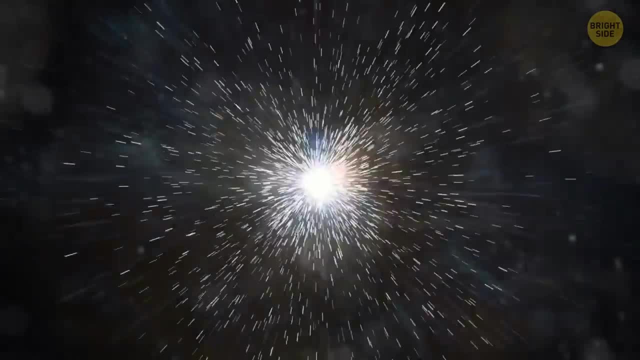 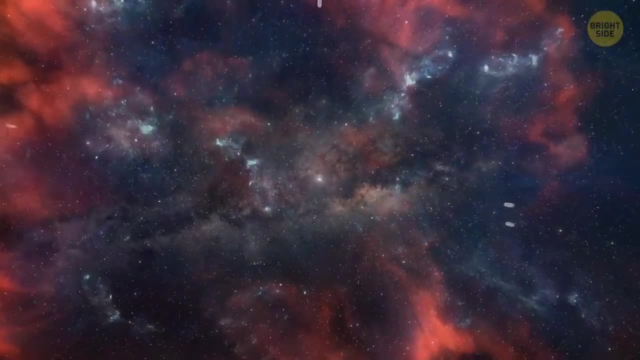 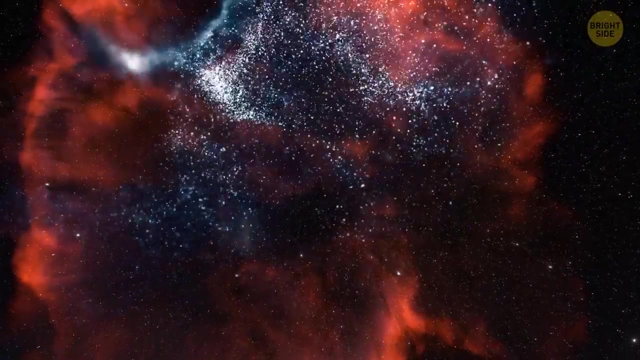 to withstand them. And here comes the Big Bang. It was an outburst of energy and matter that created everything we see now, and space, basic physical forces. It also scattered quarks everywhere, These quarks, tiny particles that make up our world. 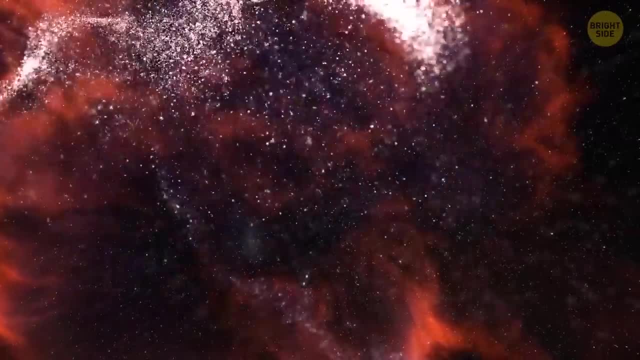 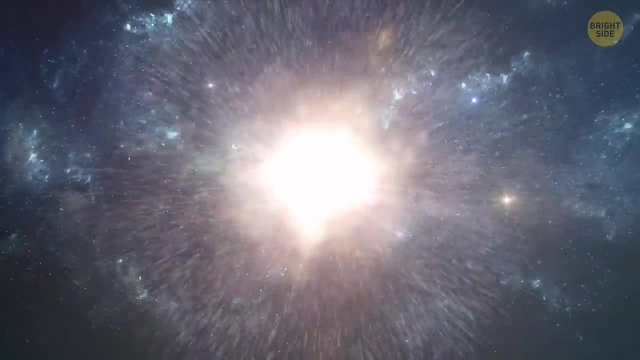 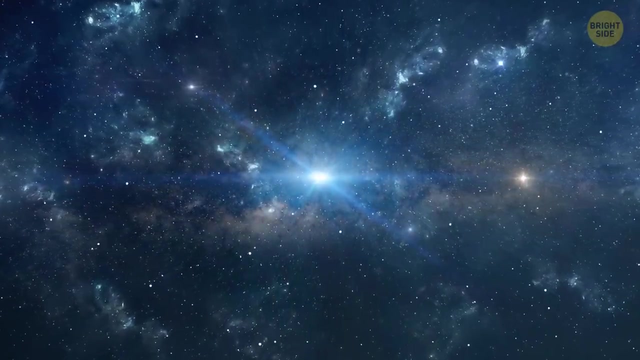 were all boiling in an incredibly hot cosmic broth. When it cooled down, gravity began to attract them to each other. They gathered into atoms, then molecules and then into the first objects, into the world stars. And all this happened just some 12 to 14 billion years ago. 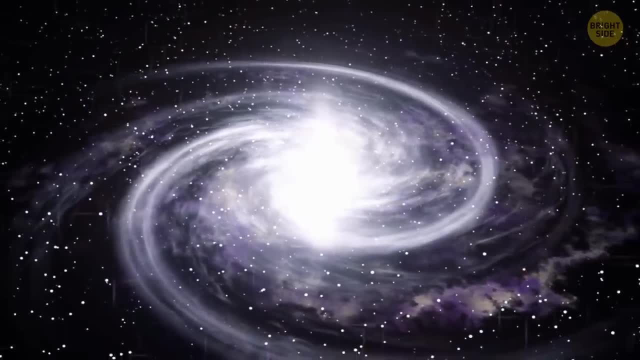 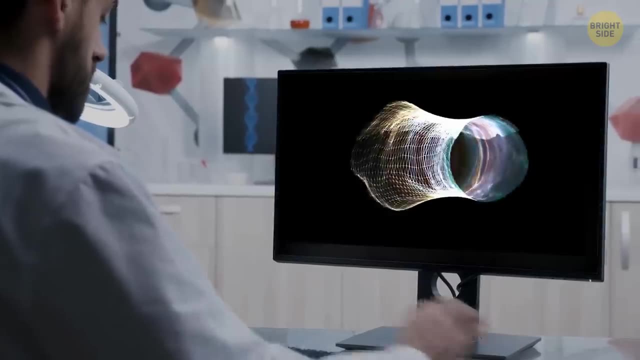 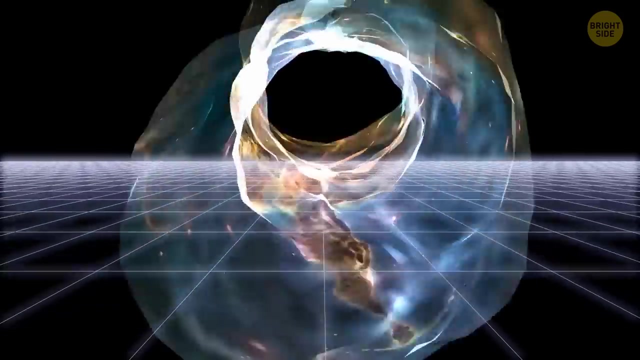 All right. now we know how our universe was created, But what was before that? Alan Harvey Guth, an American theoretical physicist and cosmologist, has devoted his whole life to solving this mystery. After learning about the Big Bang Theory, Guth found some flaws in it. 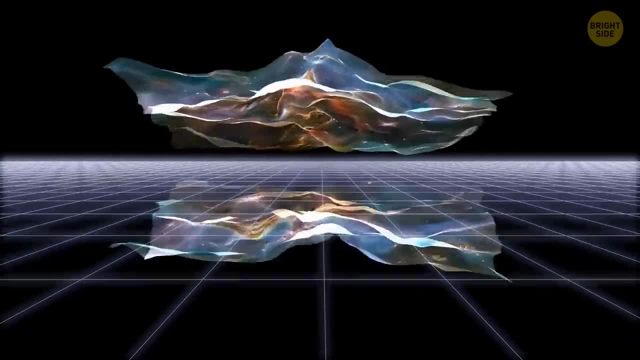 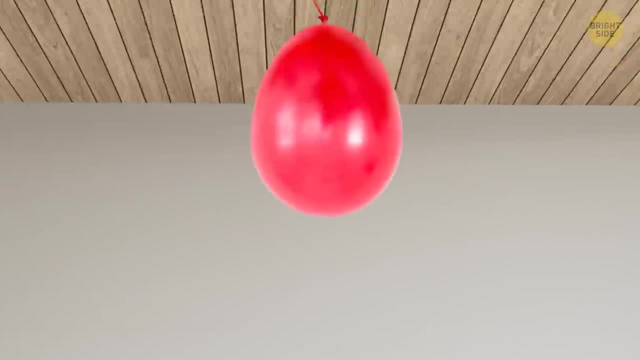 For example, the distribution of matter was very even, although it shouldn't have been. Let's hang a balloon filled with paint to the ceiling and lay a white canvas on the floor. If we drop the balloon down, it will burst. 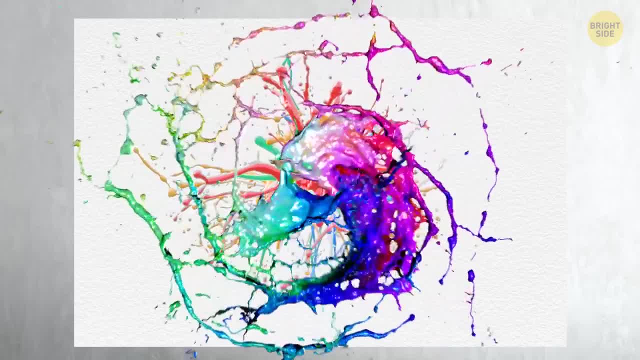 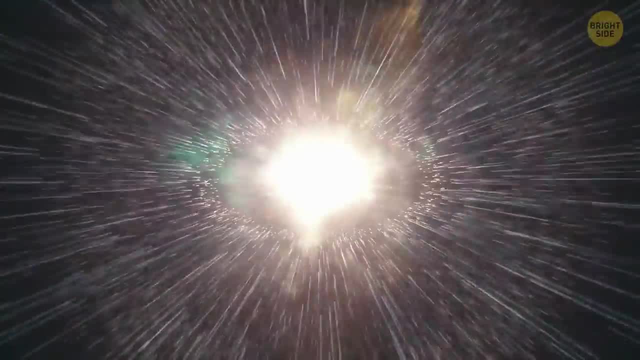 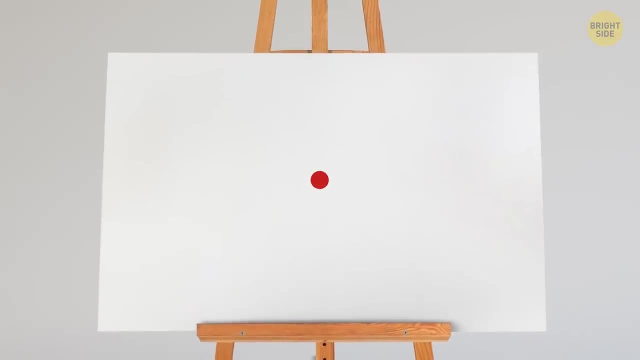 and we'll see absolute chaos on the canvas, A bunch of spots scattered everywhere randomly. Neither is like the other, But that's not really what the universe looked like. Instead of throwing a colored ball from the ceiling, let's draw a small red dot on the canvas. 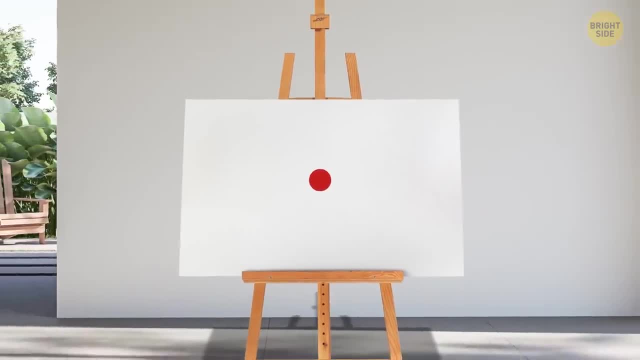 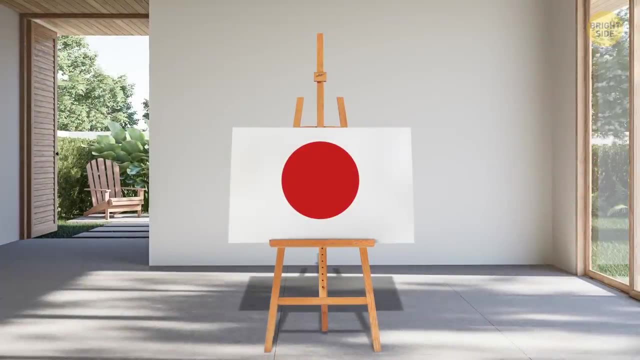 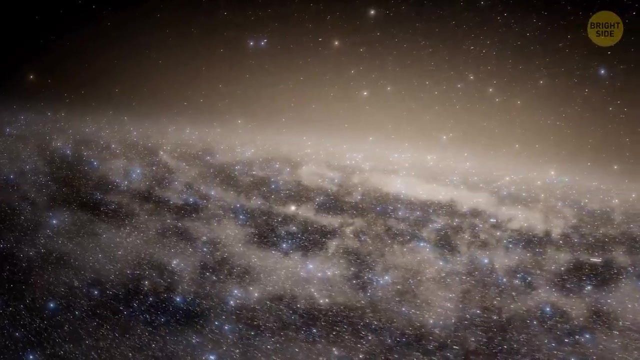 Now let's expand it a little more and more and capture this All on frame-by-frame shooting. We'll see a circle gradually growing in all directions. That's the reality. The early universe was very even and proportional. That was Guth's discovery, the theory of inflation. 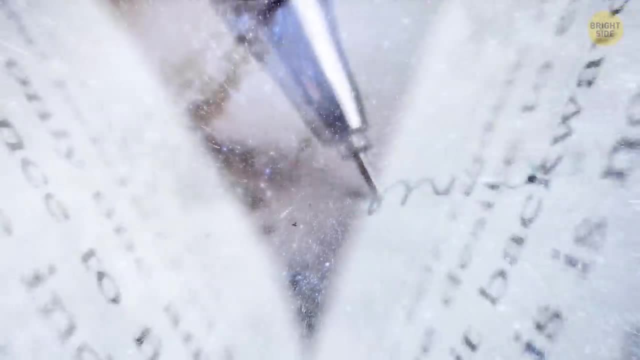 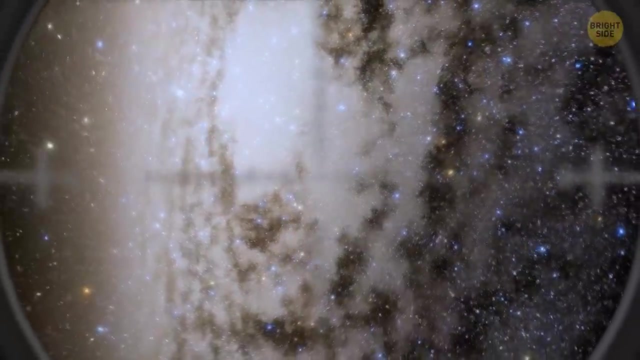 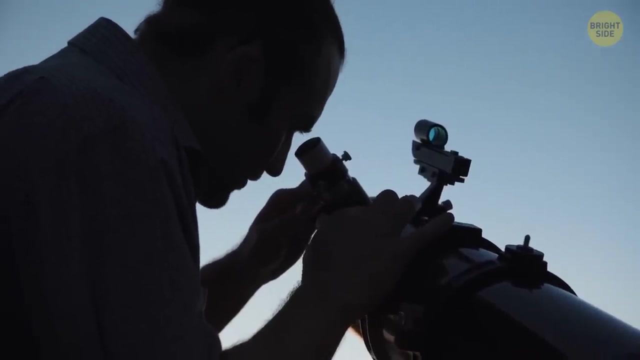 Here's what it says: Even before the Big Bang, there was some kind of force that could give the bang a strong acceleration, something that was able to distribute everything in space instantly and evenly. Guth's theory was a success, and now most scientists rely on it. 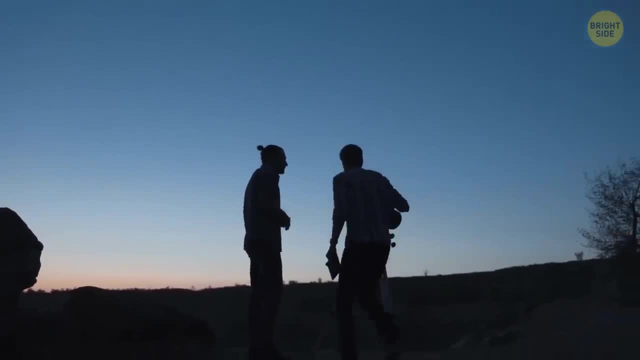 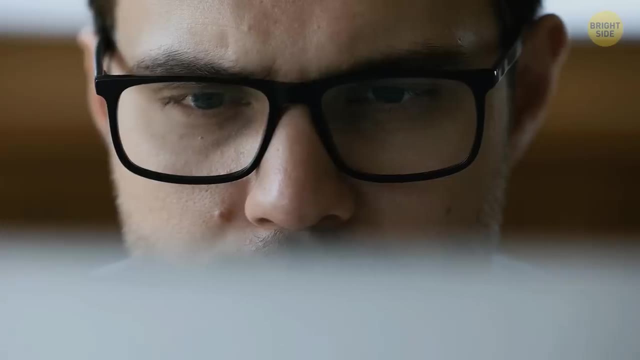 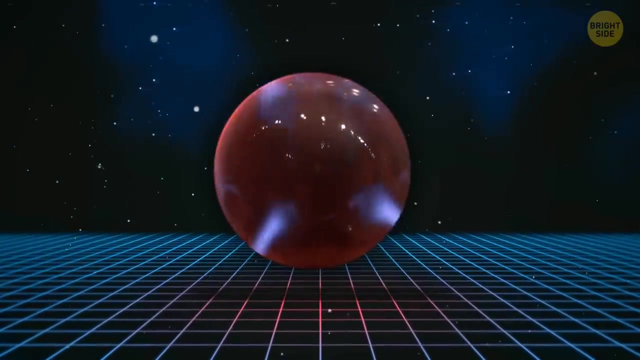 For most of them, this idea of the birth of the universe is quite enough. For most, but not for all. Martin Bojewald is a German professor of physics and in his opinion the universe was born quite differently. Remember when we talked about cosmic singularity? 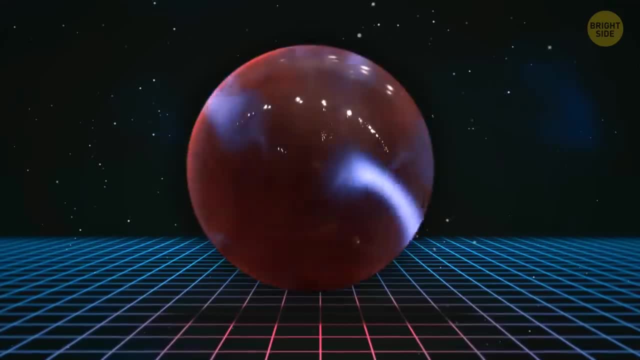 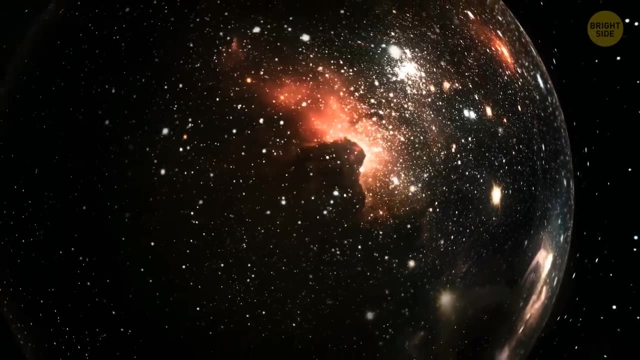 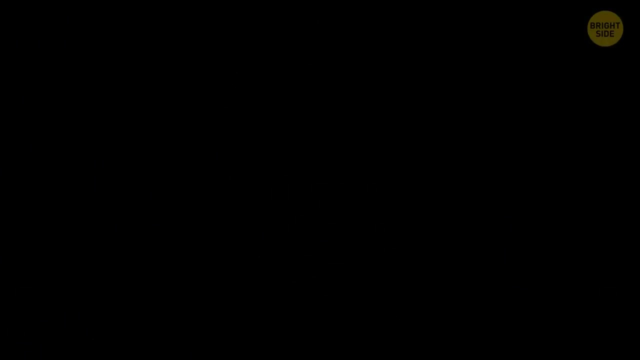 The state of the universe in which it was small, infinitely dense and super hot. According to Martin's theory, the singularity couldn't just appear out of nowhere. This is nonsense. But then where did it come from? Let's look at a pendulum on an old clock. 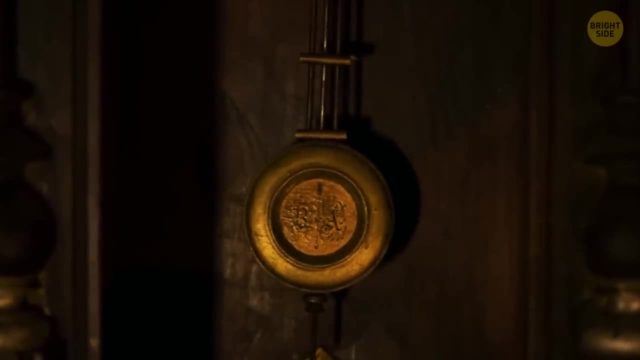 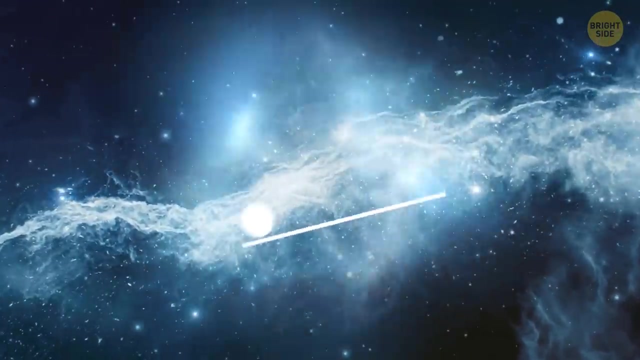 The pendulum rotates back and forth. Its movement is smooth, continuous and non-stop. This is how we usually see time. It flows and never stops. But quantum time, Ho-ho. Quantum time doesn't work that way. It's more like the second hand. 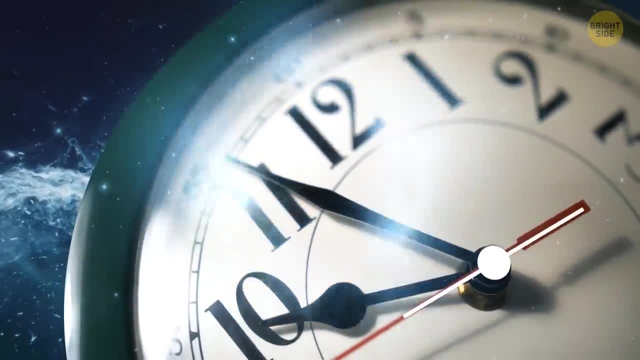 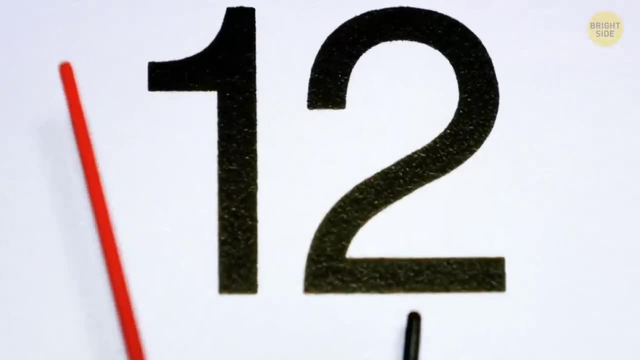 It consists of small segments and makes short pauses And, just like with the second hand of a clock, the beginning of one segment of time is always the end of another. See what I'm getting at. Let's go back to balloons again. 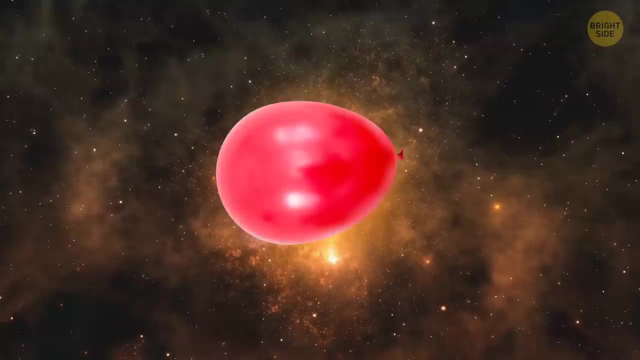 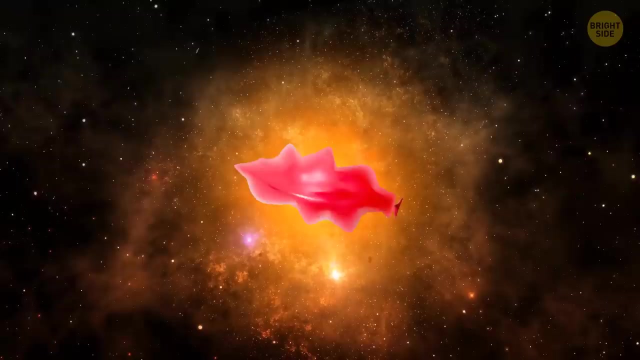 According to the Big Bang Theory, once upon a time our universe began to expand, inflate like a balloon, But sooner or later it will blow away back. The universe will start shrinking and return to the start. The universe will be in a state of cosmic singularity. 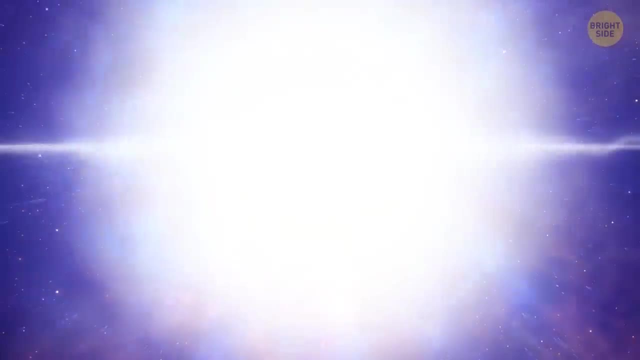 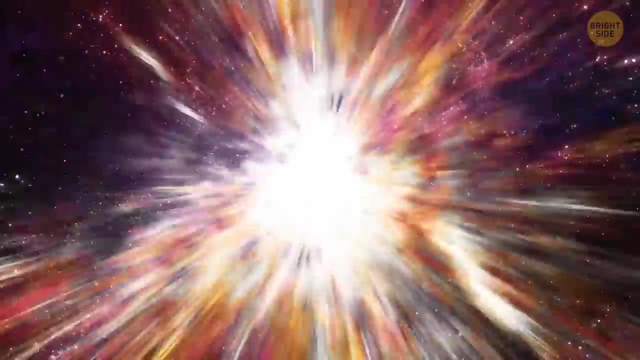 And then, guess what? The Big Bang too. Nothing appears out of nowhere and disappears into nowhere. According to Bojewald's theory, the beginning of each universe is the end of the previous one. Our universe is not at all the first. 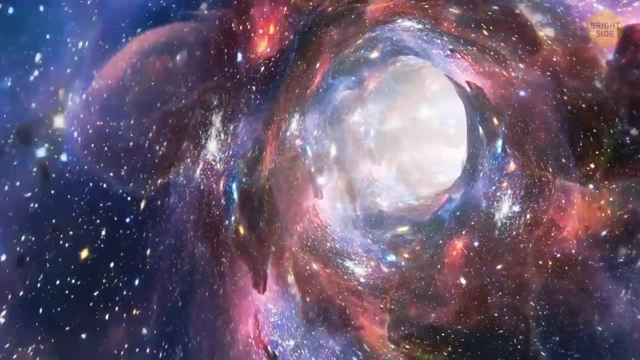 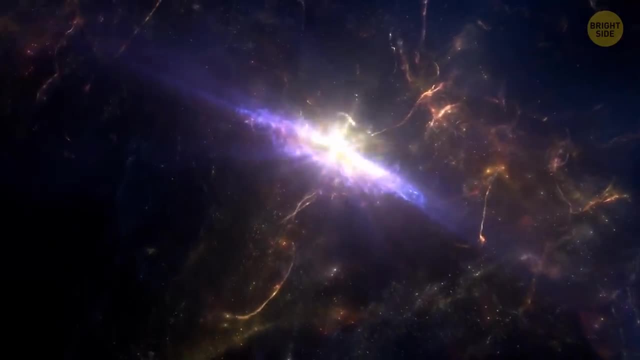 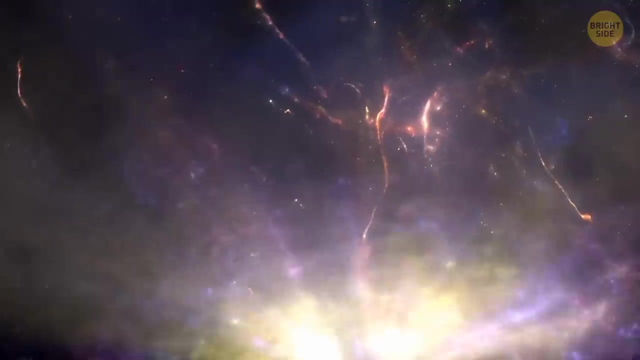 and not the last. Millions of similar universes existed before us and will exist after us. This theory, although it sounds very logical, is far from complete. Unfortunately, we don't have enough knowledge to find all the evidence for it, So for now, all this is just a hypothesis. 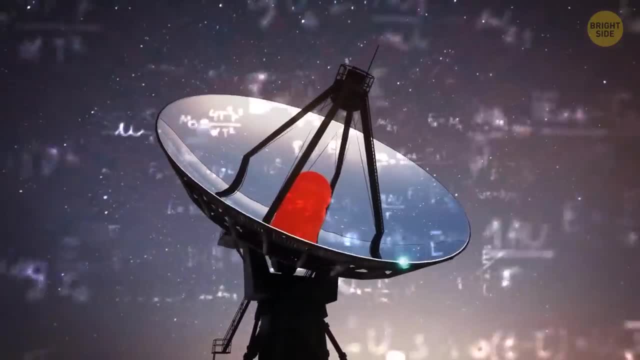 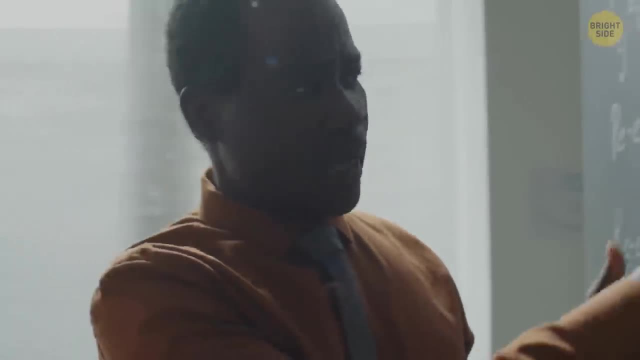 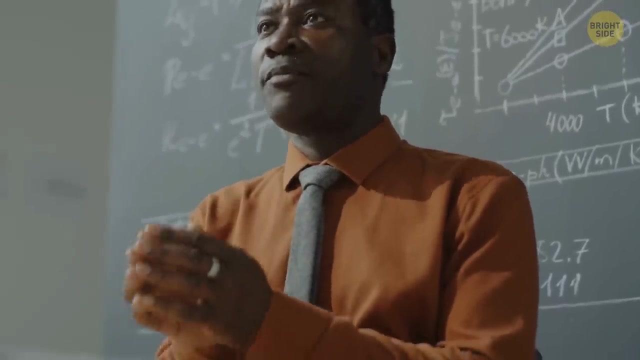 But some people come up with even stranger ideas. Scientists promote such unusual theories that no one could even think of. Neil Turok, a South African physicist, and his colleague Paul Steinhardt, an American theoretical physicist, look for answers far beyond our universe. 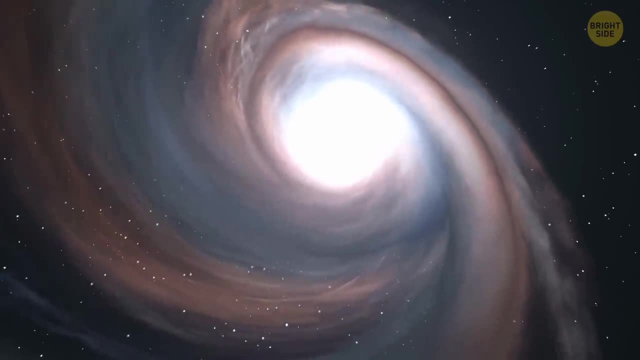 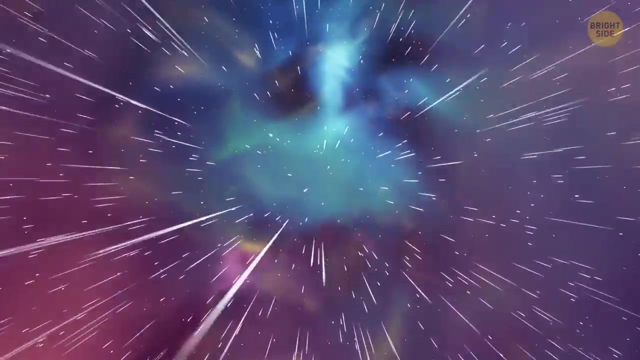 They say that, yes, our universe isn't the first one. There have been and will be an infinite number of them, And not only will there be endless Big Bangs. our universe is just one of an infinite number of others, And all of us are stuck in a cycle. 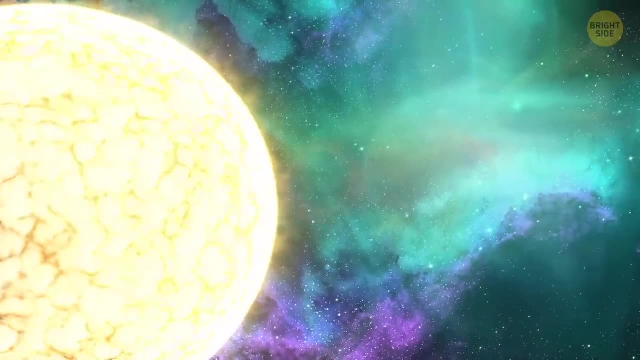 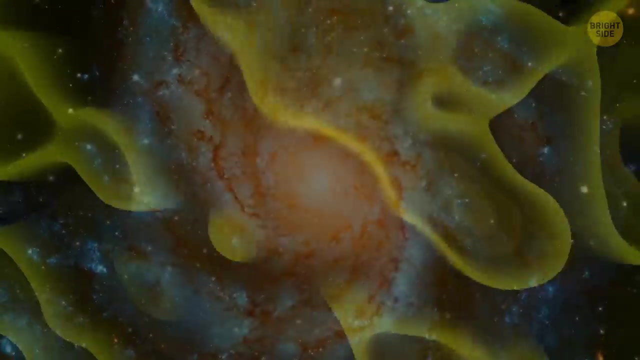 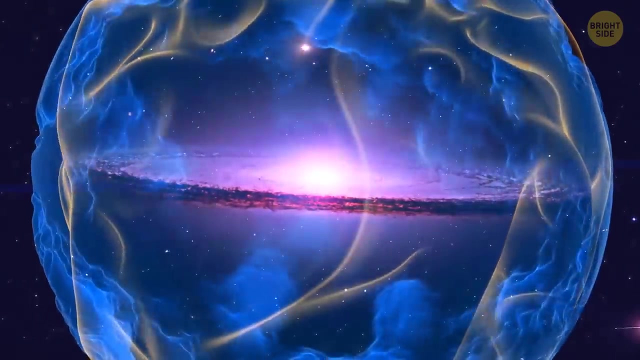 of endless rebirths of parallel worlds. This sounds incredible and frightening at the same time. But how does it work? According to this theory, our universe is located inside a soapbox, a so-called brain, as in membrane. In other words, we're stuck in some kind of elastic surface. 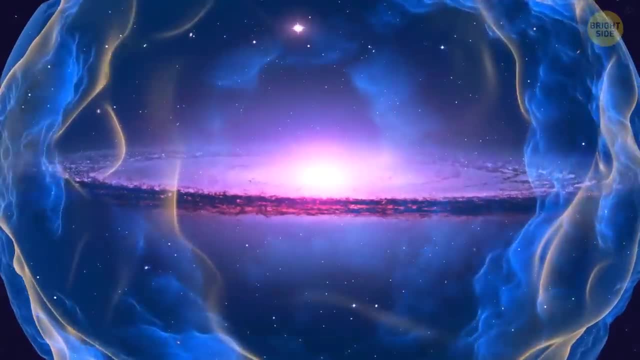 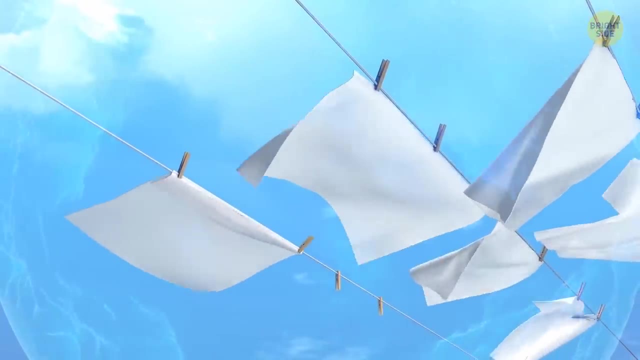 that's capable of contracting, stretching, oscillating and so on, Like pieces of fabric on a rope. these parallel universes are located near each other. Each one has a neighbor. We're not the exception. Another universe may be an inch from ours. 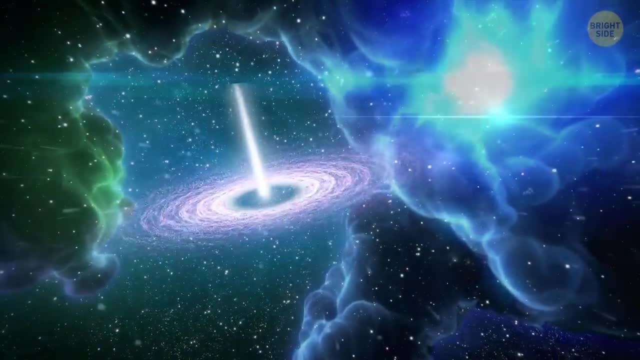 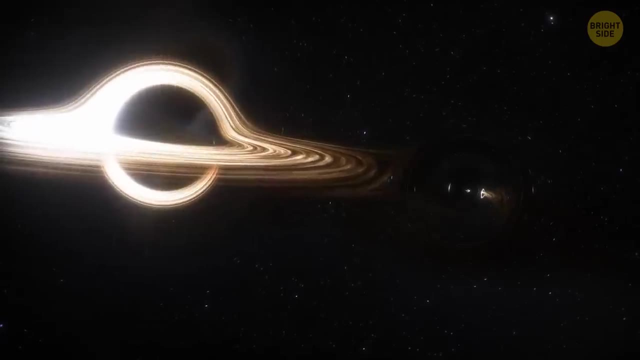 but we can't see it. That's because there's a tiny space between us, And this tiny space contains the fourth dimension. How do these universes originate? Through brain collision. These brains are getting closer to each other very, very slowly. 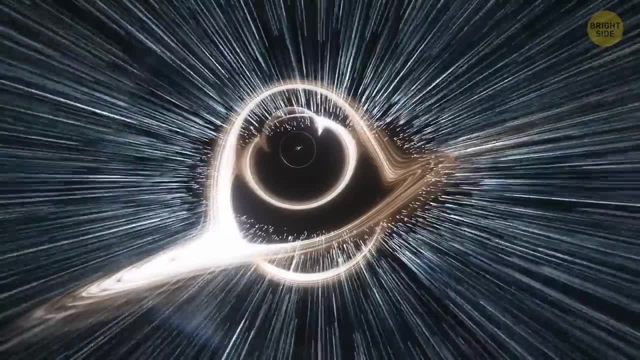 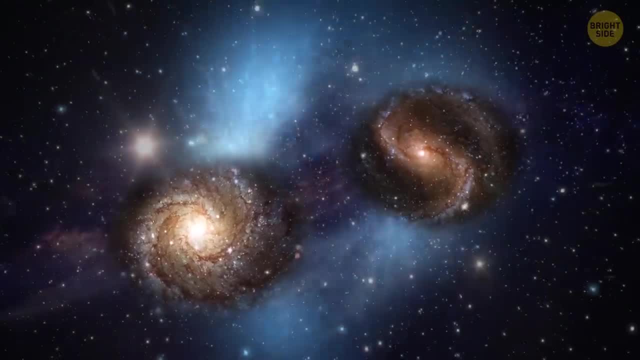 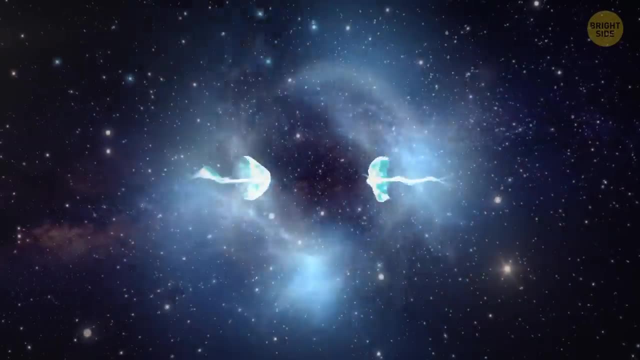 until one day they finally collide. Their collision creates two Big Bangs and two parallel universes. Then they're moving away from each other. The created worlds continue to live- We're currently at this stage- But when they disappear, the brains collide again. 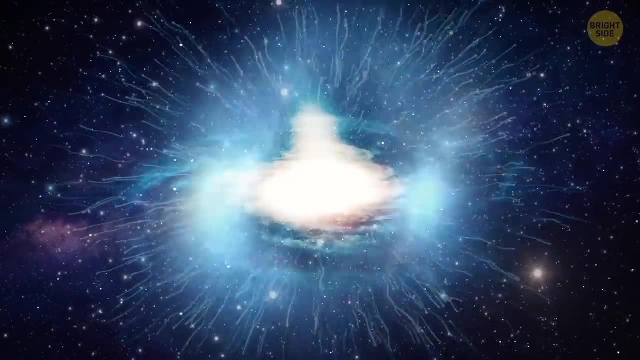 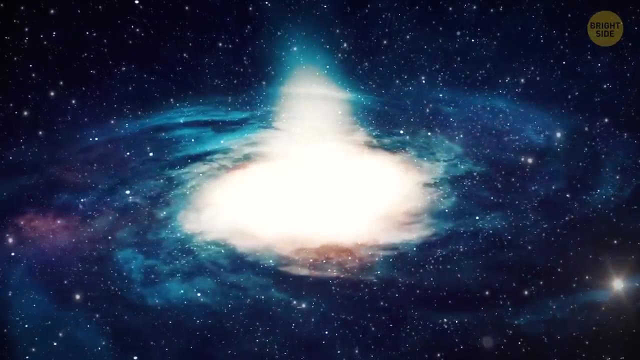 And this will lead to the birth of a new universe. Remember the inflation theory? There was a mysterious energy that pushed and accelerated the Big Bang. Well, if we did collide with another universe, that would explain everything, Of course, everything described here. 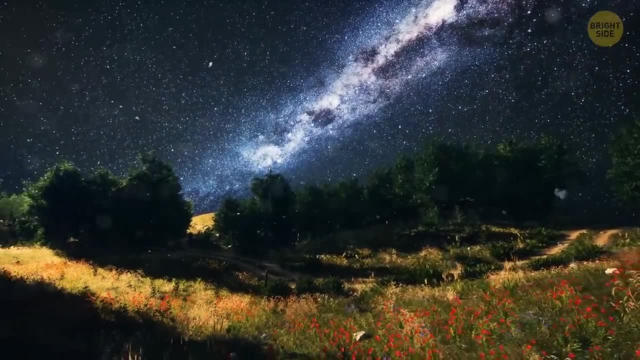 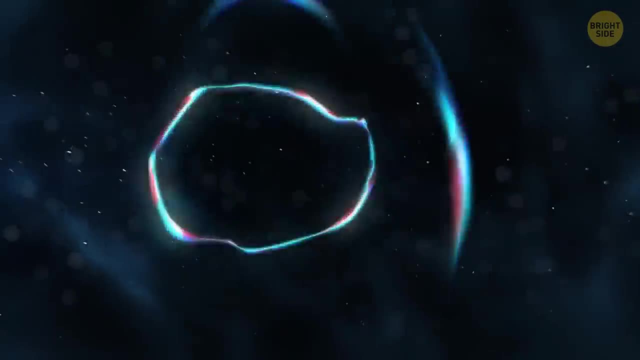 is a great simplification. When you hear that our world is some piece of fabric on a rope, it sounds like complete nonsense. But this idea is based on string theory and M-theory- two giants of quantum mechanics, If they turn out to be true. 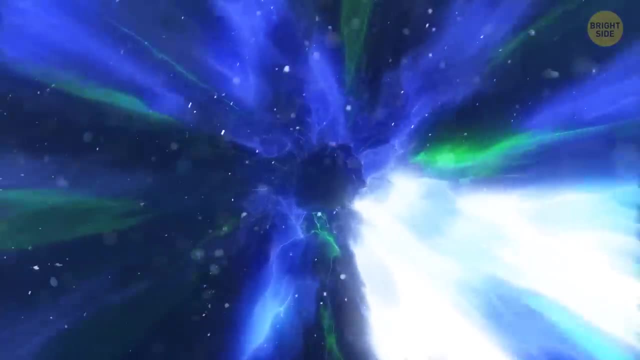 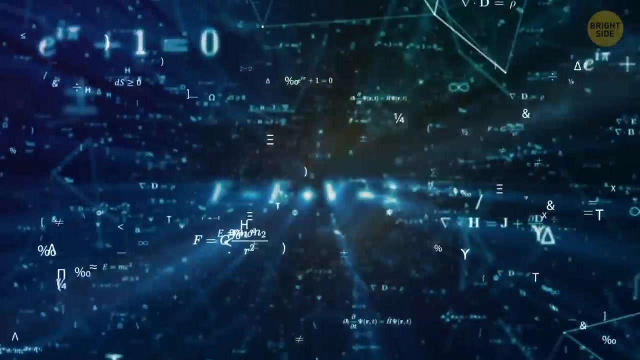 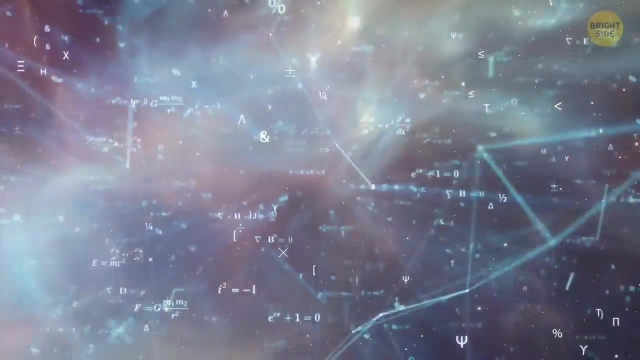 they could explain almost everything in our universe. Creating a theory is an incredibly huge process. Turok and Steinhardt made a huge amount of calculations and swept away many, many non-working theories. Also, to work this out, they have to overcome the limits of the human mind. 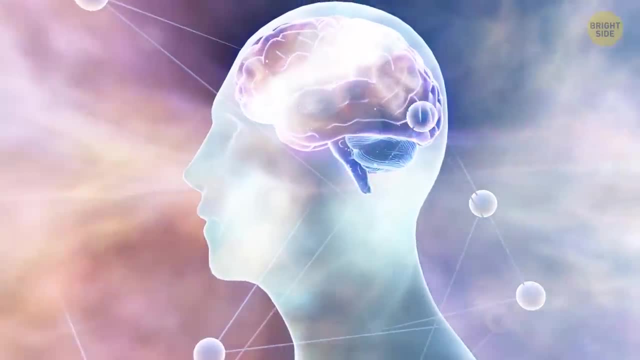 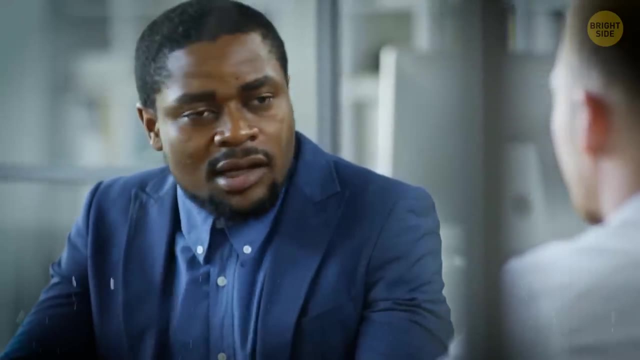 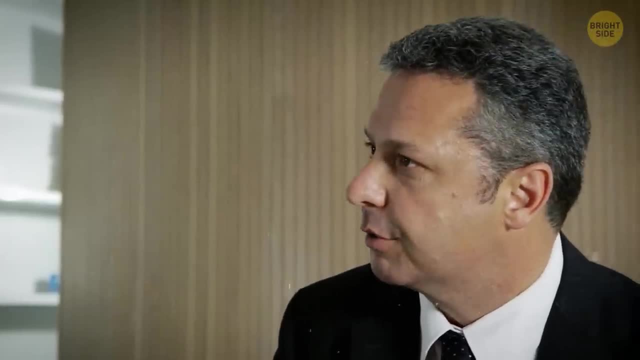 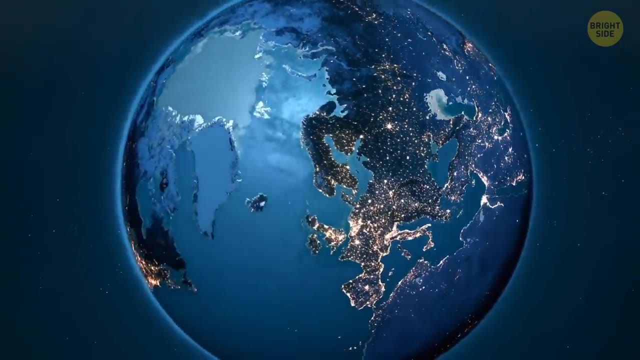 just like everyone else, They're also afraid of change and the unknown, And it's really scary to question everything we once believed in. Many years ago, people didn't believe that the Earth was round. Then they were outraged by the Big Bang theory. 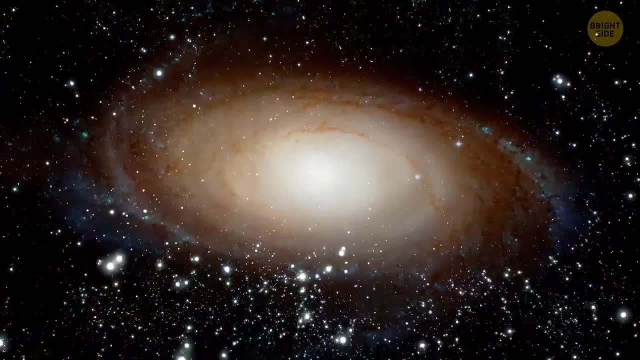 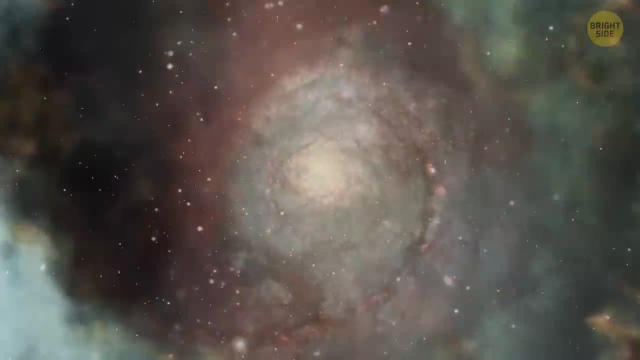 We can't make discoveries without struggle and fear. That's why Turok and Steinhardt don't plan to give up so easily. After all, the evidence that we have now only says that each of the three theories is equally possible. So which answer is correct?